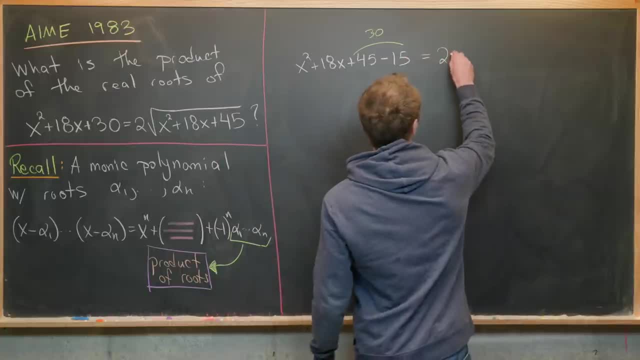 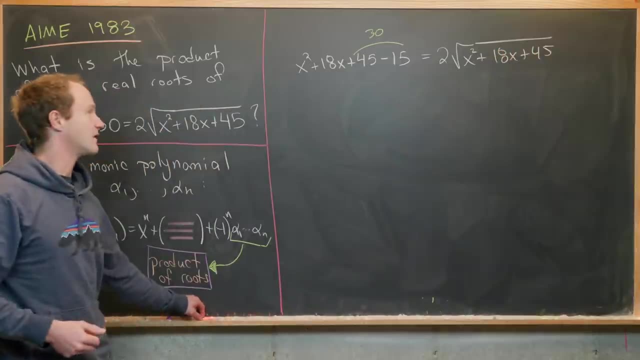 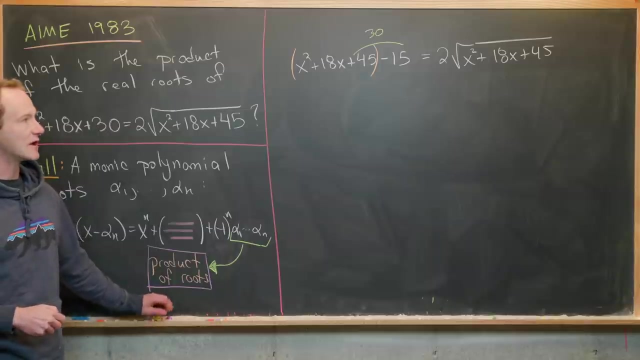 And then we can leave the right hand side as is. So we've got x squared plus 18x plus 45.. Next we can think about grouping the x squared plus 18x plus 45 on the left hand side and rewrite it as the square root of x squared plus 18x plus 45, quantity squared. So let's do. 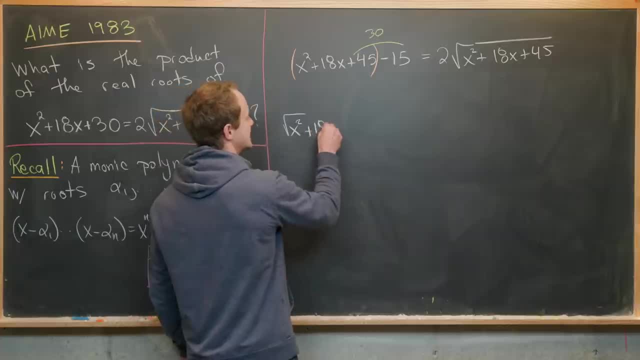 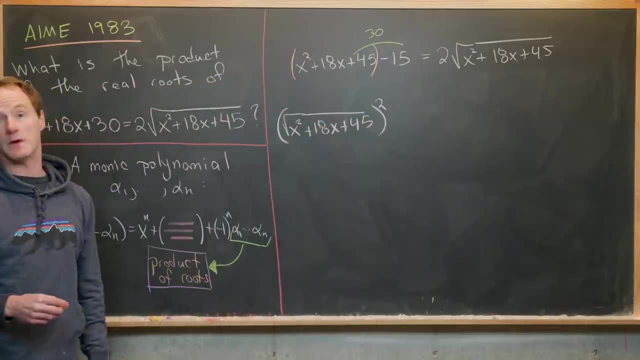 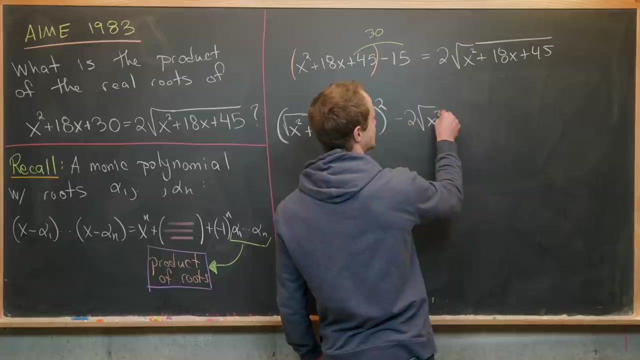 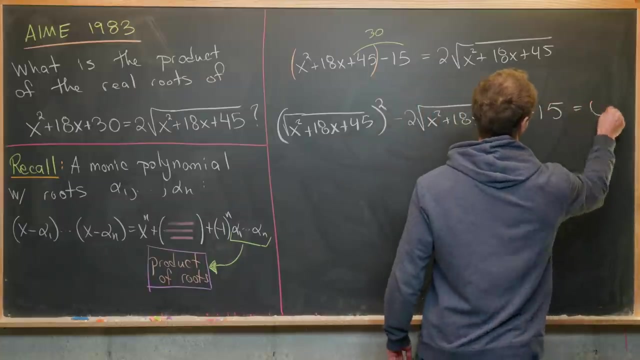 that. So we've got the square root of x squared plus 18x plus 45, quantity squared. So we got that from this thing with the peach parentheses, And then I'm going to move this over. then we have the square root of x squared plus 18x plus 45.. And then finally, minus 15 equals zero, But notice. 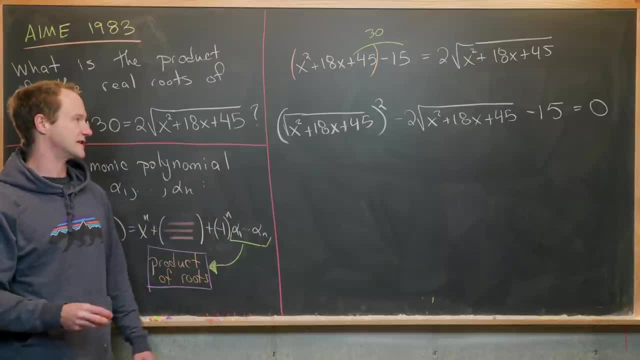 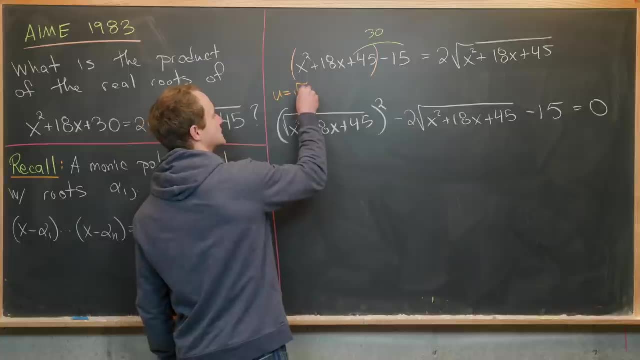 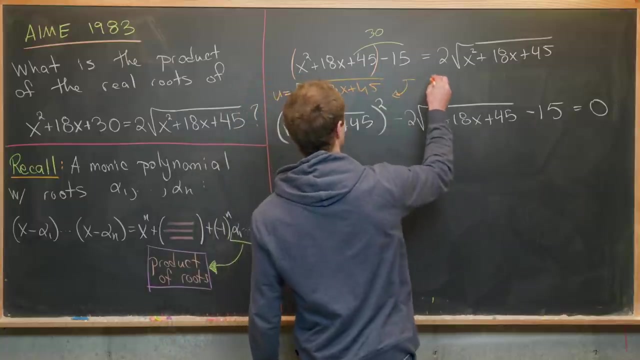 that looks like a quadratic polynomial where the variable is the square root of x squared plus 18x plus 45. So in fact we could just let u equal the square root of x squared plus 18x plus 45. And notice that this polynomial is really u squared minus. 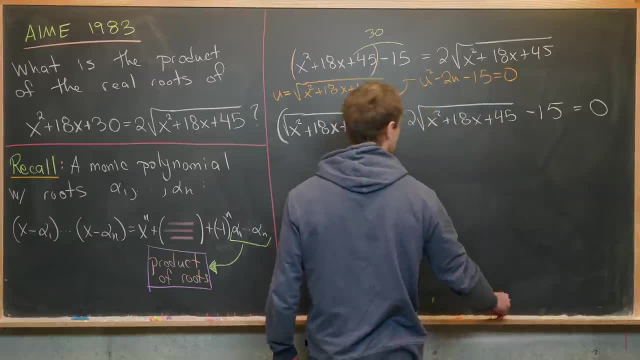 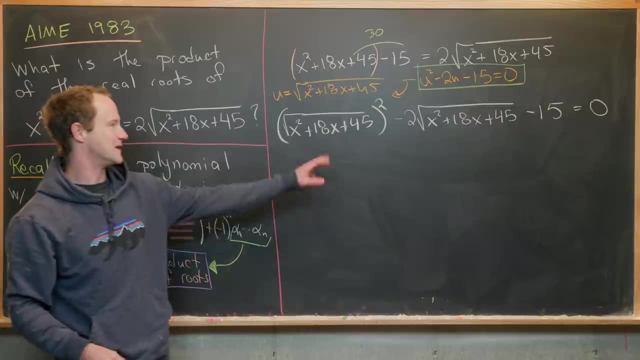 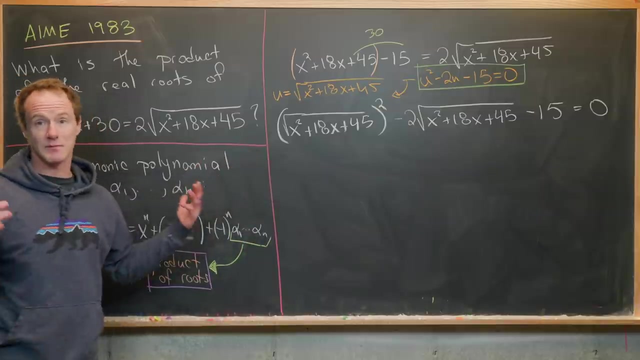 2u minus 15 equals zero. We're actually not going to make that substitution because it's not super necessary, But if you want to rename this big object- you know some other simpler variable- that's okay. Okay now, being inspired by factorization of quadratic polynomials. 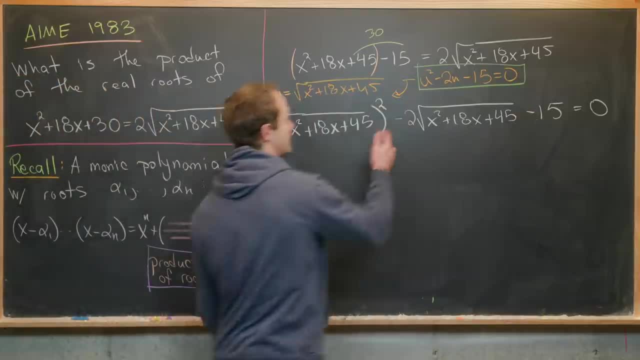 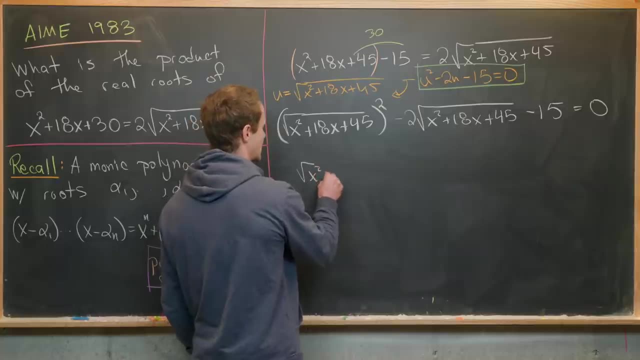 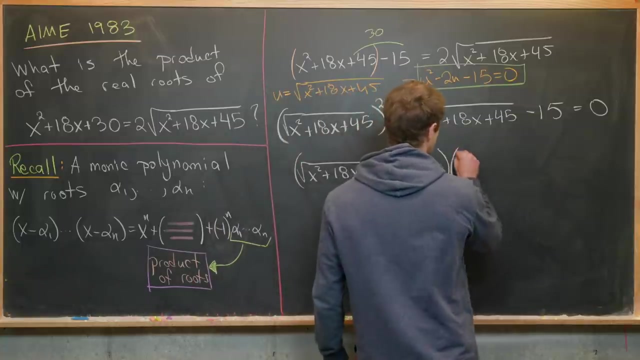 we see that negative five and three multiply to negative 15, and they add to negative two. So that'll give us a factorization of this thing. So we have the square root of x squared plus 18x, plus 45, minus five times square root of x squared. 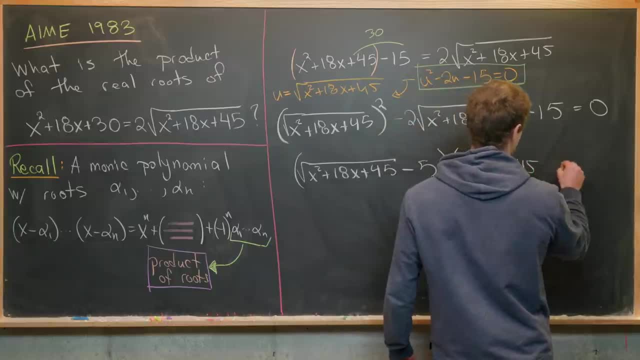 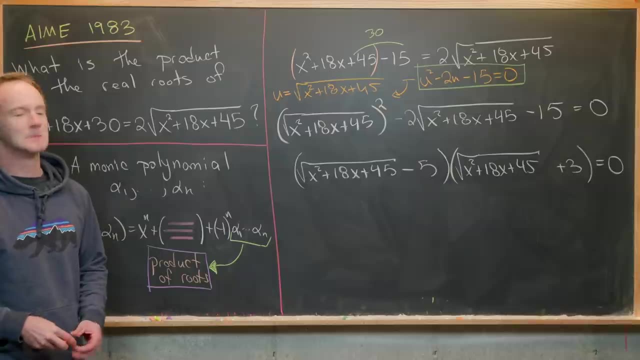 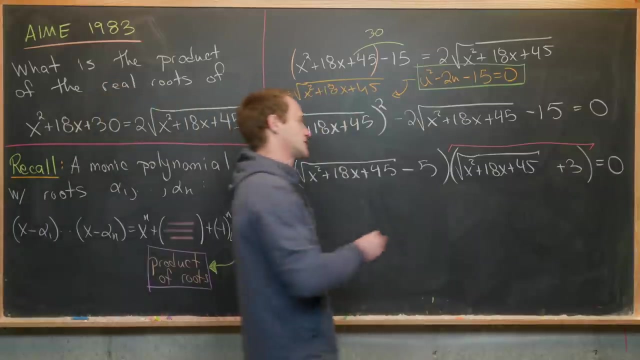 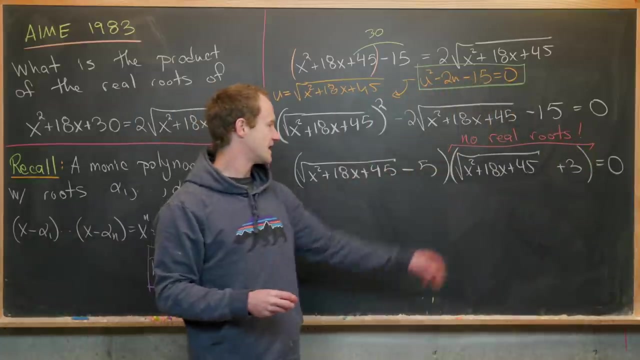 plus 18x plus 45 plus three equals zero. And now we want to carefully look at this And notice that this second factor does not contribute to any of the real roots. So let's just put no real roots from this factor. And that's because the square root of x, squared plus 18x plus 45, plus three, is: